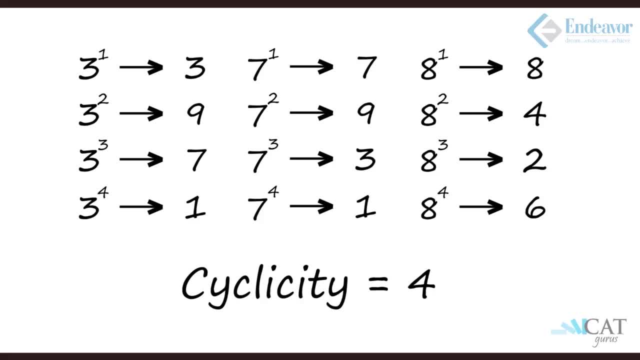 8. These are numbers which alternate on every 4.. Let's see how it happens. Let's take, for example, 2 to the power 46. So every 4 times it's alternating. So if we remove all the multiples of 4, say 44,, so 2 is left. So 2 to the power 2, which is 4, that will be the. 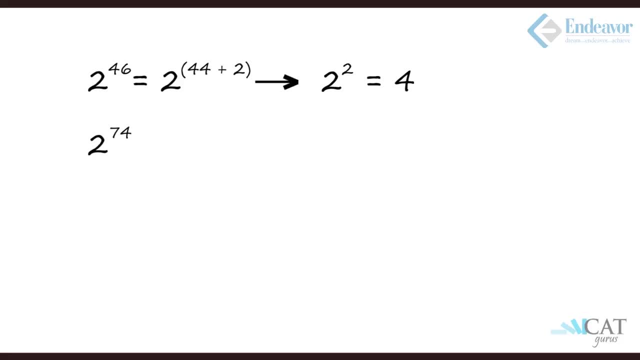 last number, Say 2 to the power 74. So let's remove all the multiples of 4.. So 72 is the highest multiple. If you remove that, 2 is left. So 2 square again is 4.. Let's do it slightly more technically. 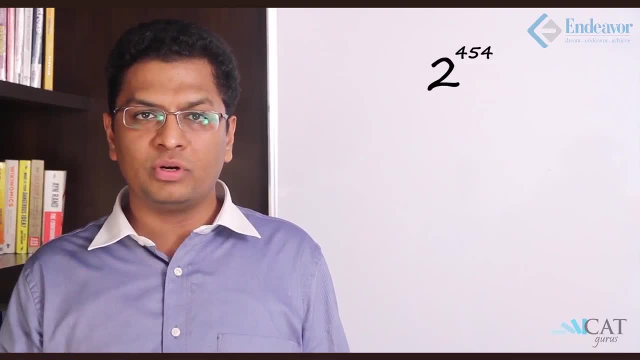 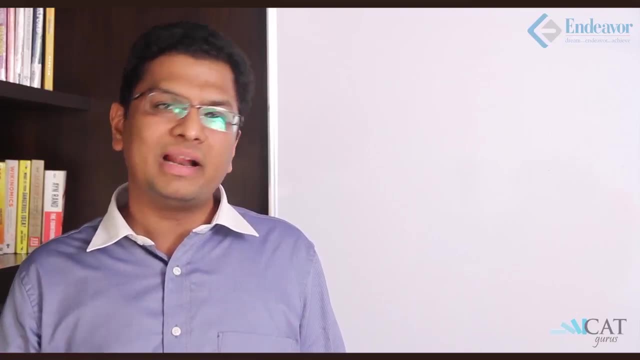 Say 2 to the power 454.. So 2 to the power 454.. Now let's divide it by 4.. So 454 divided by 4, the remainder is 2.. Hence it will be 2 square. What happens if it's 2 to the power? 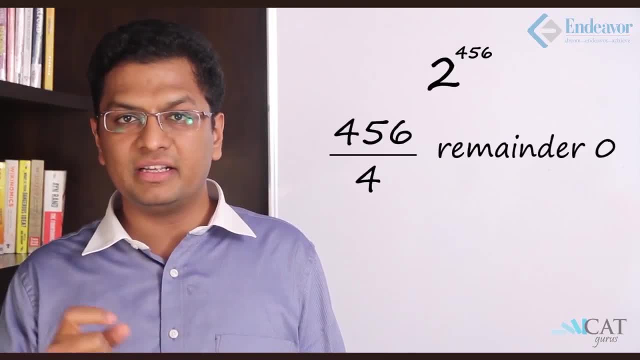 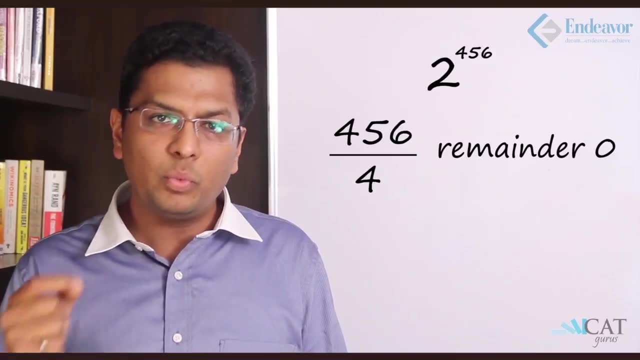 456?. It is perfectly divisible by 4.. The remainder is 0. But technically, can you ever have a remainder of 4?? So 2 to the power 4 will never come across, which here is equal to 2 to the power 0. So if it is 0 as the remainder, then 2 to the power 4, which is 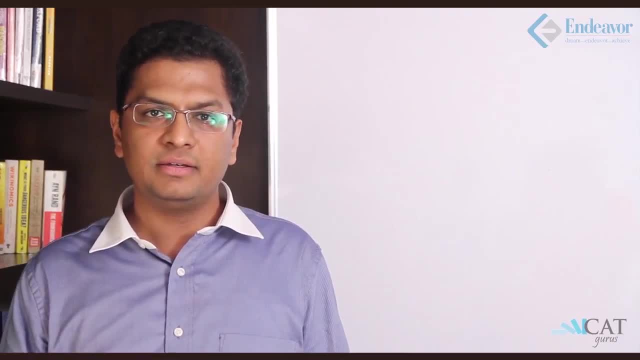 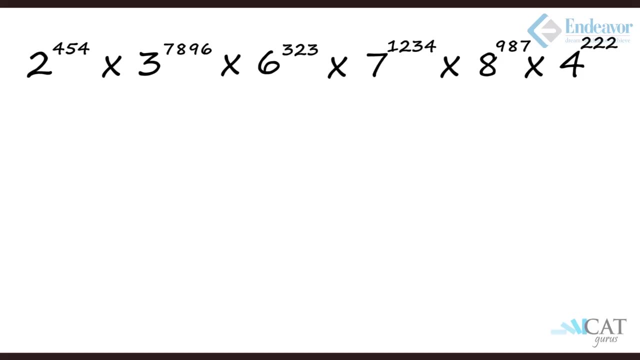 2,, 4,, 8 and 6.. 6 will be the last digit here. Let's put it back into the original equation that we had 2 to the power 454 into 3 to the power 7896 into 6 to the power 323 and. 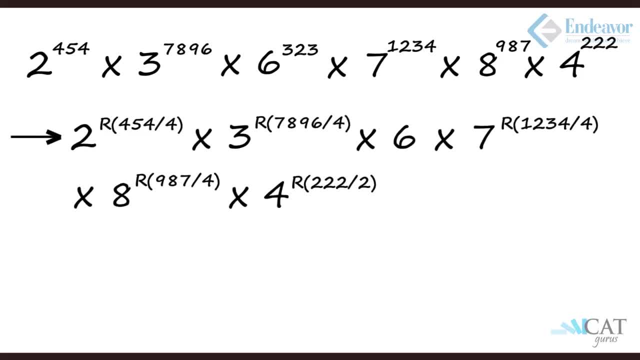 so on. So 2 has a cyclicity of 4.. So we divide 454 by 4.. 3 again has a cyclicity of 4.. 6 does not have cyclicity, It is constant. Let's keep it. 6 simply. 7 has a cyclicity of 4.. 8 also has a cyclicity of 4.. And 4 has 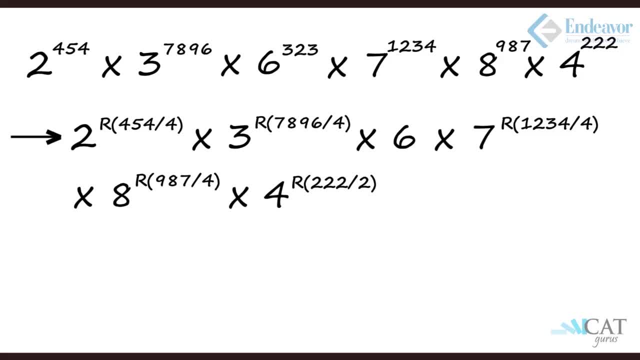 a cyclicity of 2.. In case of 4, what do we do? It's either even or odd. So let's go back 2, square into 3, square into 6, into 7, square into 8, cube, And it's 4 to the power. 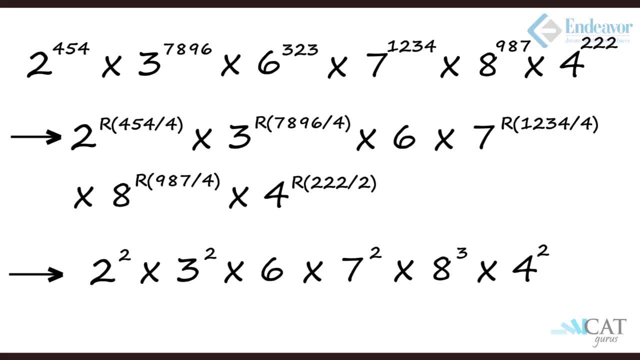 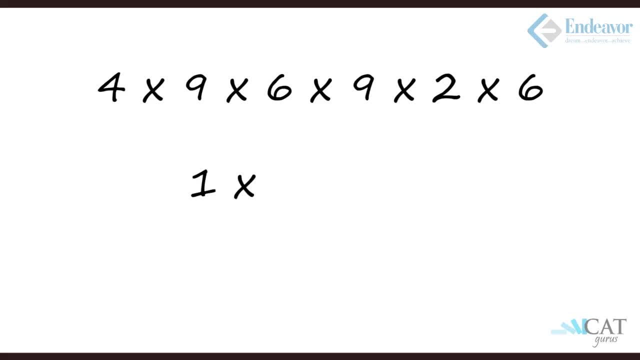 2.. So we get the last digits as 4, 9,, 6,, 9,, 2, 6.. Let's multiply: 99 is 81.. So 1 is there. So we can rule it out 6 is 36.. So it's 6.. 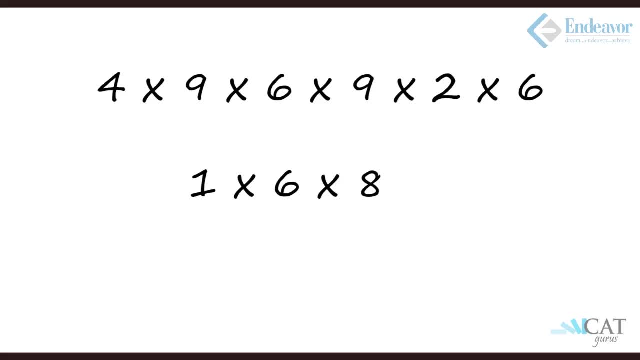 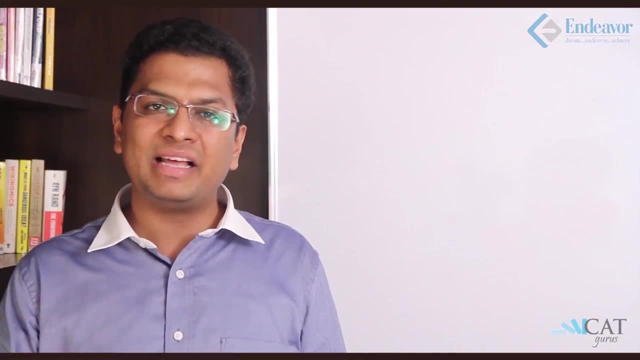 Let's put it one place: 4 into 2 is 8.. So 6 into 8 is the final answer, which is nothing but 8.. So the last digit of such a huge calculation is 8.. This is how we can apply the same thing.